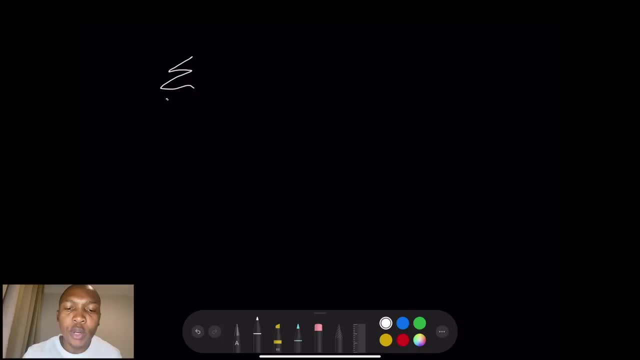 something. So we've got a counter. Now sometimes they would say: let's say the counter starts from 1 up until 30 or 1 until n. Now you consider if the counter shows you the number of terms that you would have in that particular series right Now, and then you have the general. 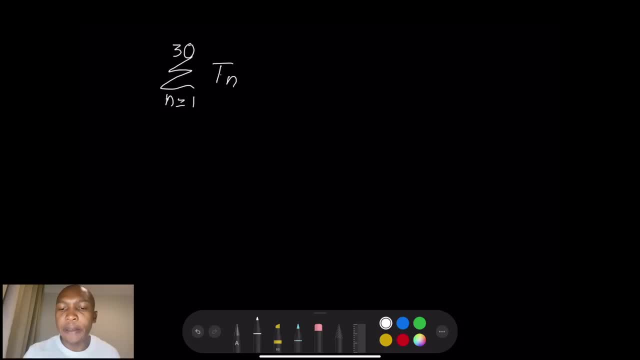 expression, which is, let's call it, tn. here You'd have the general expression, and the general expression would give you the- you know the terms that are, yeah, the terms in the series. Okay, So you must just keep in mind. sometimes you would have a counter. Let's. 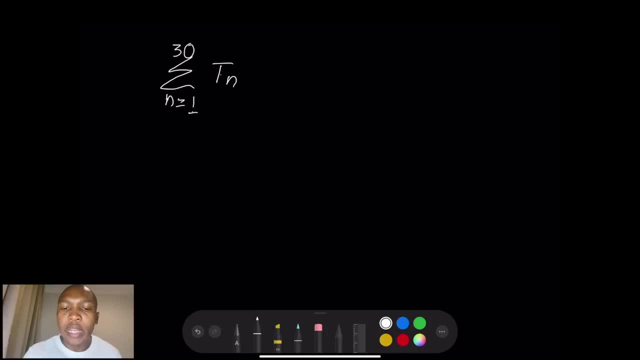 say, in this particular case, our counter starts from 1 up until 30, right? So it means that you'd have term 1 up until term 30. Okay, So how many terms would you have? You would have 30 terms. 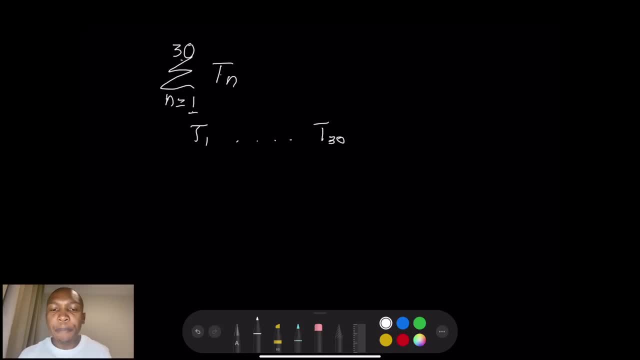 Obviously you'd be counting from 1 up until 30. But if, for instance, you've got a counter, let's say: let's say it's k is equal to 3 up until n. Okay, So let's say n. 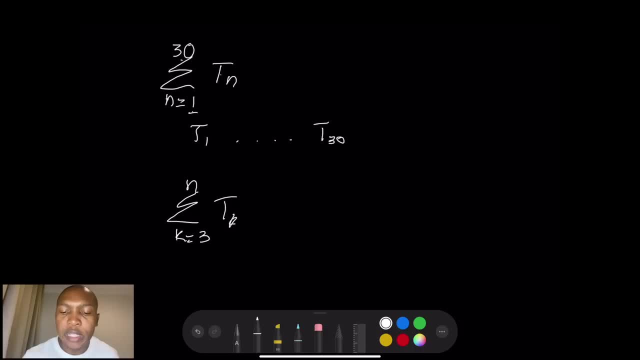 number of terms. And we've got an expression there: tk. Right Now. you would imagine if we started from 1, you'd be talking about n number of terms, But in this particular case, you are not starting from 1.. You're starting from 3, right? So how? 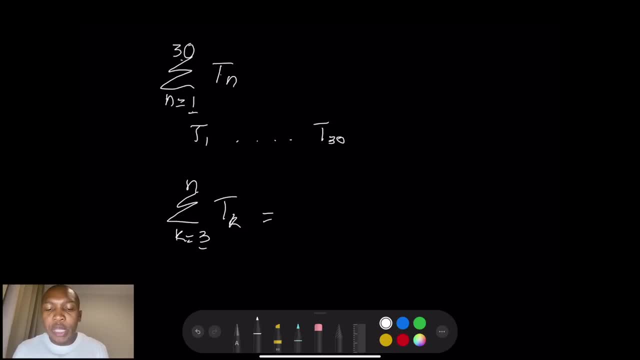 many terms would be missing. It means that you're missing 1 and 2.. So essentially, your term 3 is your term 1.. I hope you get that right. So in this case we're missing two terms. So it means: 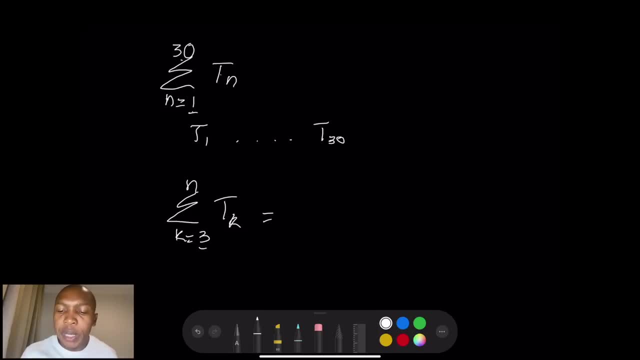 that the total number of terms should be, in this particular case, n minus 2.. Okay, Because you're missing the first two terms in a sense. Okay, So just keep in mind that that counter is very important in order to tell you you know how many terms you have in that series. All right, 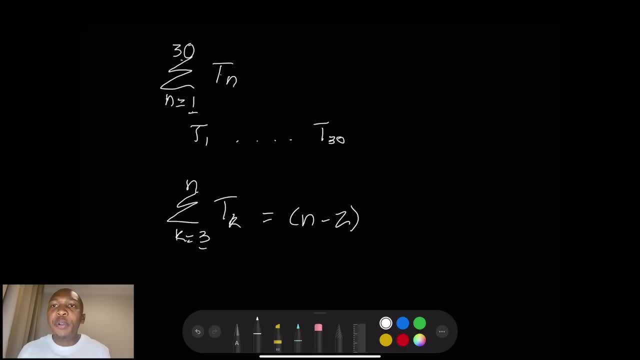 Without any further ado, I think let's jump into examples so that I show you how to go about navigating this particular part. Okay, All right, Let's start with our first example. So they've given us there's: the sum from k is equal to 1 up until 30.. And we've got our general expression. 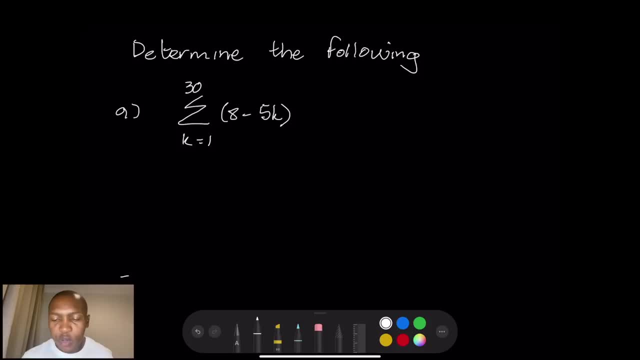 right there. So what I'm going to do is just. you know, I have to learn to use different color variations, just to show you what I'm trying to do. So first of all, let's find out what are the terms that we 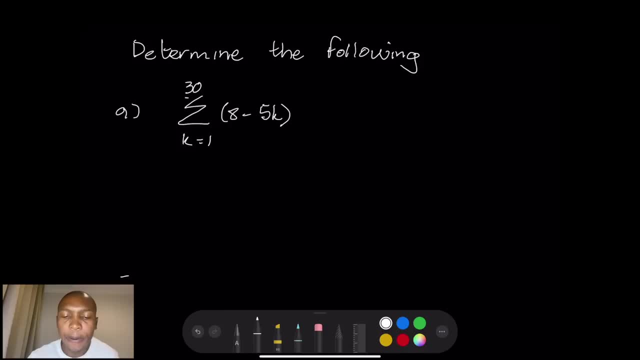 have. Look at our counter. It's starting from 1 up until 30.. Okay, So in this particular case, we know we're starting from 1.. We're going up until 30.. Okay, So we're going to make sure. 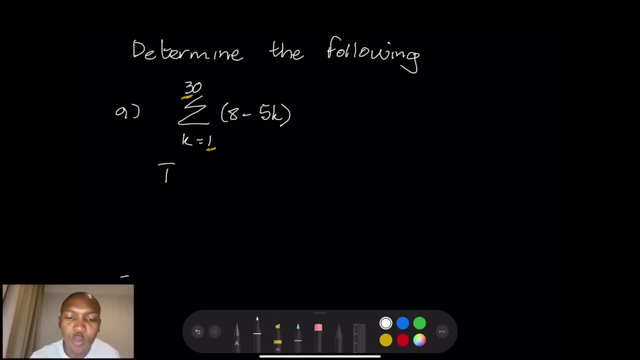 that we get the first term, So t1.. In this case it means we're going to substitute 1 into that expression. there 8 minus 5k. So there's our expression. So we're going to just make sure that we substitute for 1.. And then we're going to 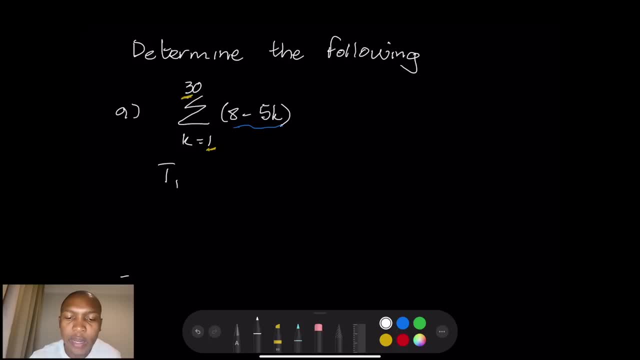 increment as we go. So we want term 1.. So that's going to be 8 minus 5 multiplied by 1.. So that's 8 minus 5 into 1.. And what about term 2? That would be 8.. 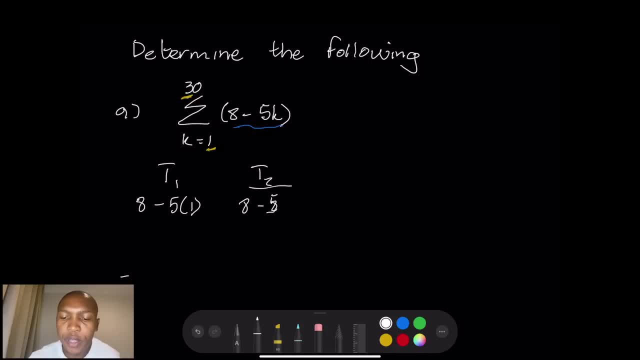 Minus 5.. Sorry, 5 times 2.. Okay, And let me just erase that So that doesn't disturb us. Okay, So that's 8 minus 5 times 2. And obviously, term 3, that would be 8 minus 5 times 3.. Of course, 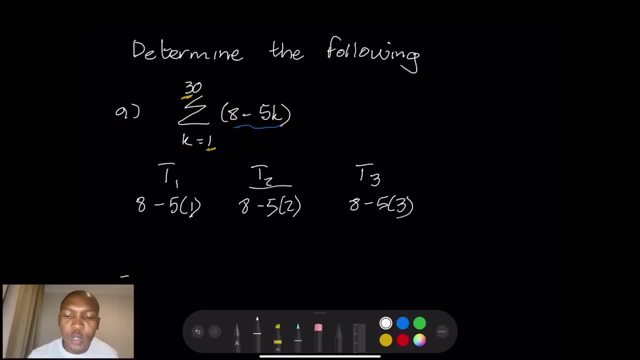 if we started from 2, you'd start substituting 2 there and 3 and 4, and you'll increment as in that particular order. All right, So 8 minus 5, that would give us 3.. So that's. 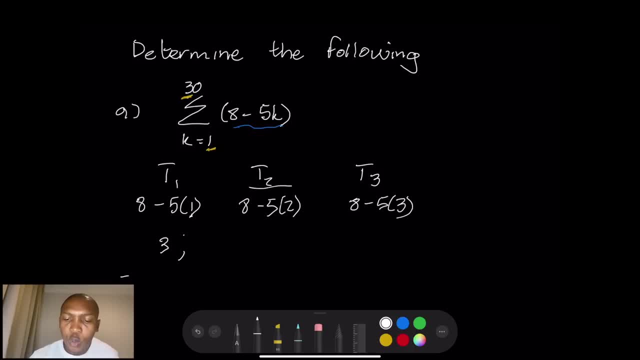 our first term: 8 minus 5 times 2. That's 8 minus 10.. That would be minus 2.. And the third term, that's 8 minus 5 times 3. That's 8 minus 15.. And that would give us a negative 7.. All right, 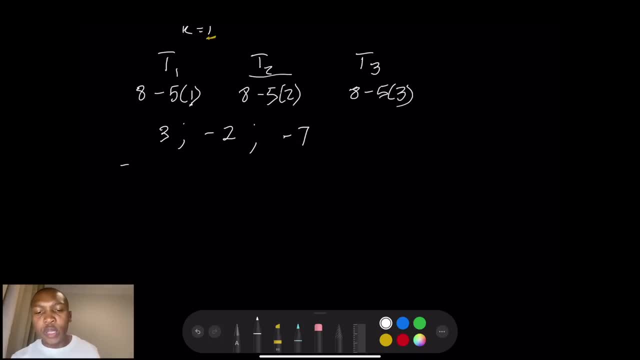 So now here's our sequence. So we need to find out first what type of a sequence it is Okay. So if I look at it, let's take. okay, let's take the difference there. So if you look, if I look at that, 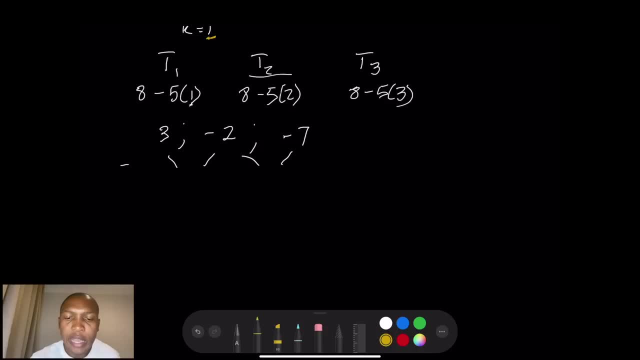 the first difference: 3 minus a negative, 2. In fact, no term. 2 minus term 1. So that's negative. 3. So that would give me negative 5. Agree, So negative. 7, once again, term 2, term 3 minus term. 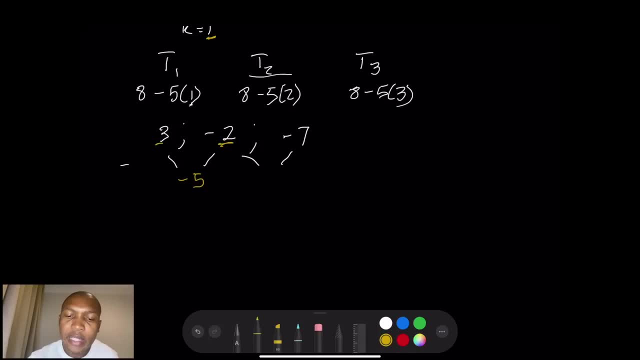 2, negative, 7 minus a negative 2. So you should be careful there. So that would be negative 7 minus a negative 2. So obviously a negative times a negative becomes a positive there. So you end up with minus 7 minus a negative 2. So that would be negative 7 minus a negative 2.. 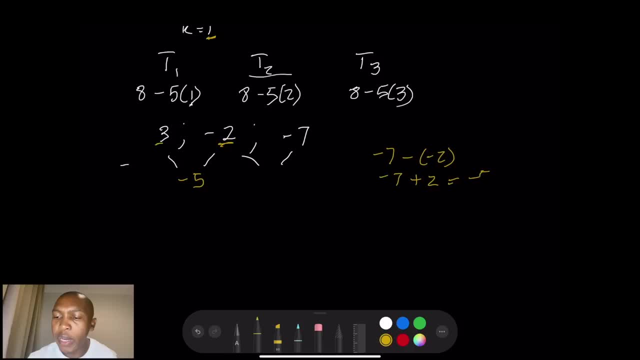 So you end up with minus 7 plus 2, which also give you a negative 5.. Okay, So we know that in our sequence we've got negative 5 as our common difference. So definitely, this is an arithmetic sequence, All right, So remember what is the sigma notation telling us? It's telling us we. 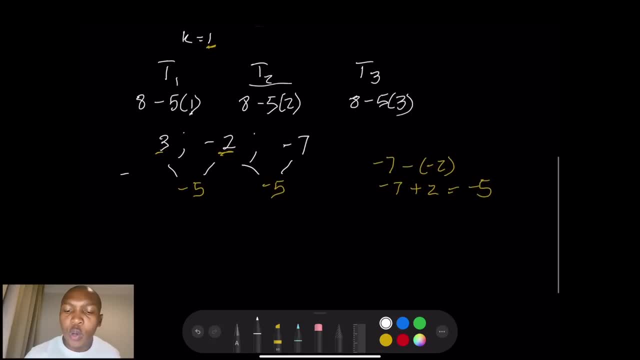 must get the sum. Okay, So in this case, we know how to get the sum, So it means that we would get the sum. So, in other words, I'm going to have to stand in front of my partner as long as there is. 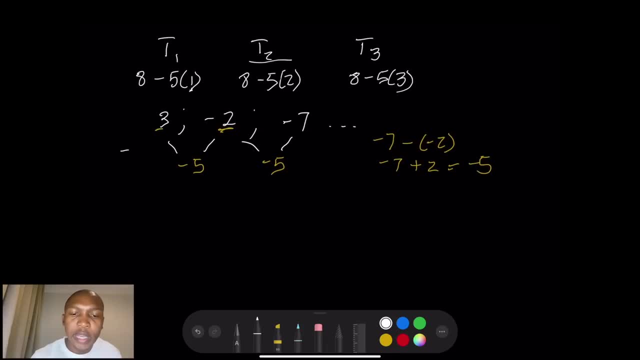 no additional in their value. Next time we're going to increase that value, we must also see which value to be given out. However, you cannot have negative 4 minus negative 4, because that'll make it happen that we're actually going to have negative 5 plus a negative 5 minus. 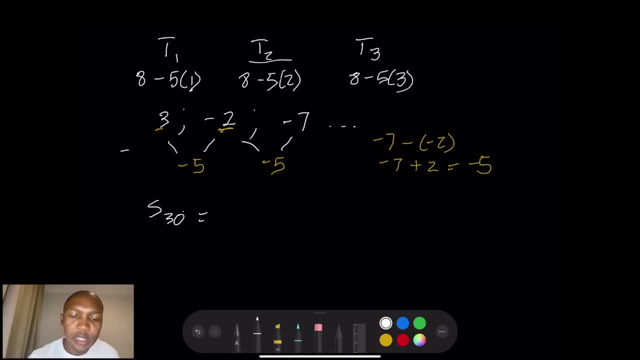 equal to um. in fact, let me just write the, the formula um, you know, as an expression first, rather the formula just in the general form: okay, so we've got sn. okay, so we've got sn is equal to n over 2, n, 2. okay, that's 2 a plus n minus 1. 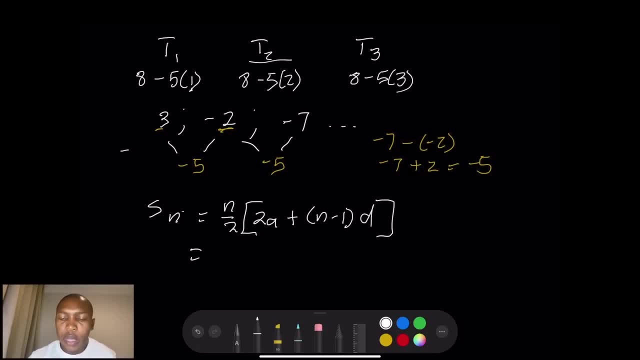 times d. okay, so, uh, just keep in mind, that's our formula for the sum of an arithmetic sequence. we know this is an arithmetic sequence. we've got a common difference. so we're going to write the formula for the sum of an arithmetic sequence. so now we're looking for s 30. okay, perhaps i should make my brackets a little bit different. 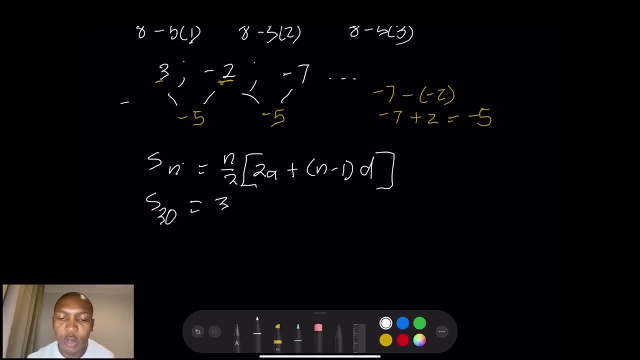 so that it's visually appealing. okay, so this is going to be 30 over 2, okay, uh, let's make that blue. all right, i hope that's still visible. uh, into 2 times. our a value is 3. okay, so there's our a value there. 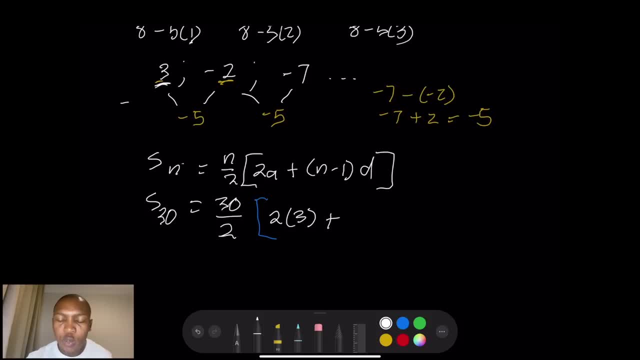 uh, plus, so that's n minus 1. remember, n is 30, so that's going to be 29 multiplied by um. in this case, we've got a minus 5 as our common difference. okay, and we close that bracket. okay, that's our blue bracket. so in this case, let's: uh, just quickly get that into the calculator, okay, uh, there's my. 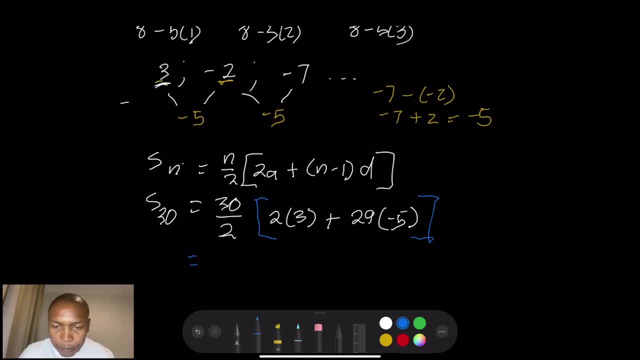 calculator there. all right, so, and we get a value of. so that's 15, um, and i seem to get a value of negative. okay, so let me just go back to the white. so that's negative 2085. so the sum of the first 30 times is 2085. okay, um, i think. 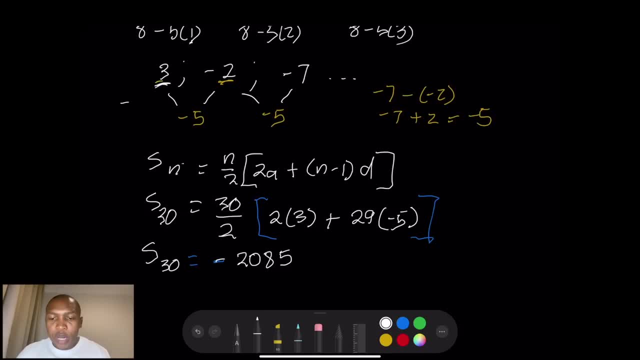 that is that, okay. so i want us to quickly jump into another one. all right, all right, uh. looking at our second example, so there we've got another um expression that is given to us. so we are taking the sum there and our counter this time does not start at one. uh, it starts at two, and you should just be careful. 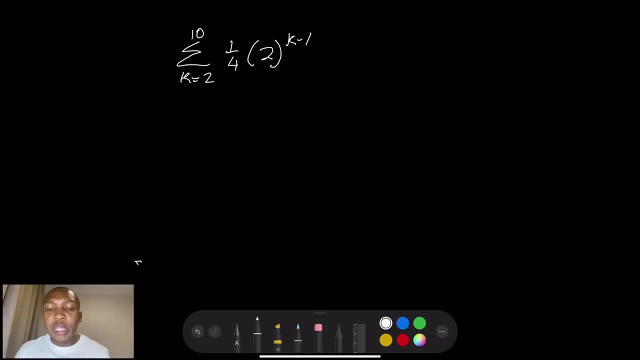 sometimes the counter starts at zero, and what that means is that you're going to add, you know, just another. so if it's from zero to two, you're going to have to add another one. so if it's from 10, obviously that would be 11 terms. okay, um, because you're not counting from one, but you're. 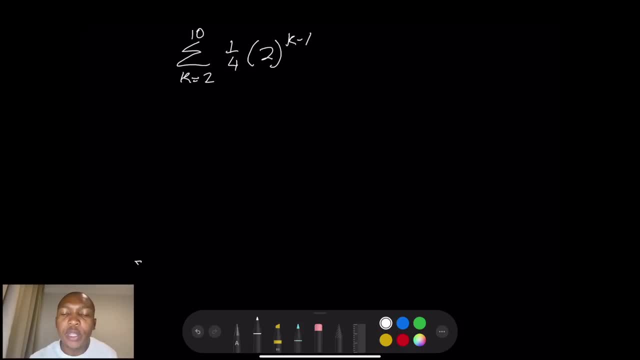 counting from zero. okay, so in this case, we're counting from two uh till 10. uh, obviously, you know. it means that we would have nine terms in this case, right? so let's start with term one, term two and term three, and for term one, we've got one over four. 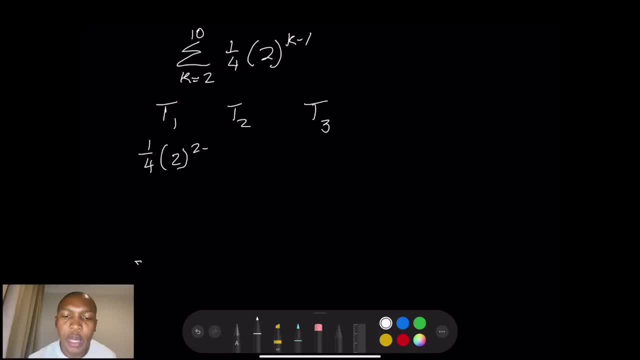 into two to two minus one, so that's two minus one. and then for term two, that's one over four, into two, that's two. um, sorry, that's uh three. uh, remember, we are incrementing now, okay, um, and one over four, that's two into uh, four minus one. and 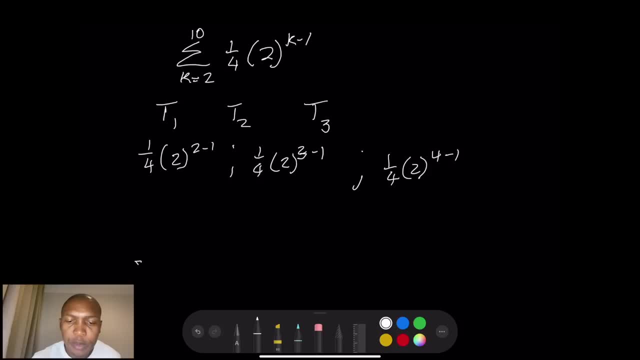 but i get there. so one over four times two minus one, that's two. okay, i mean that's one. so one over two time one over four times two. that would give me, um, one over two. so that's the first term, okay, and here i've got. 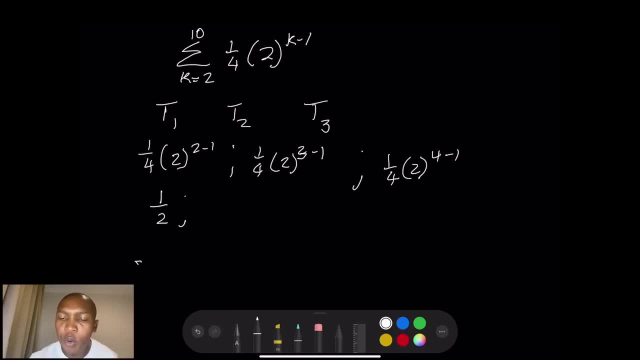 one over four times two to the power three minus one. three minus one is, uh, two, so that would be two squared, okay, which is four, four times one over four. that will give us one, okay, and um, of course, the last one, that's one over four multiplied by two to the power four minus one. 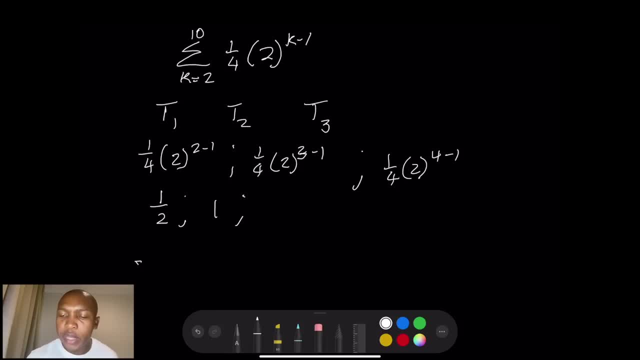 four minus one is three, and two to the power three is uh eight. so eight times one over four, that would give me uh two. so those are the first three terms, and i realize this time- and this is not an arithmetic sequence, but uh, look at this, uh. term two: 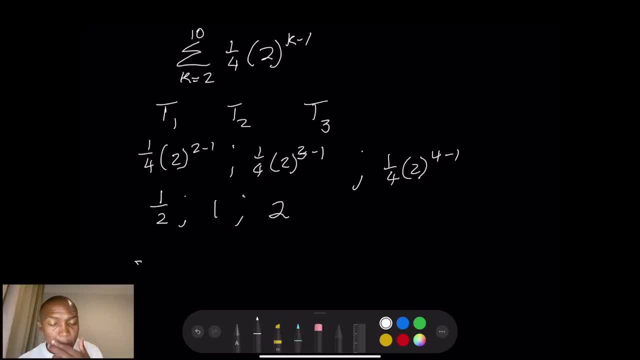 which is one divided by term one. uh, in this particular case, this is going to give us two. but also term three, divided by term two gives us two. so we've got a common ratio. okay, uh, let's do that quickly. so we've got a common ratio there and our common ratio is two in each case. 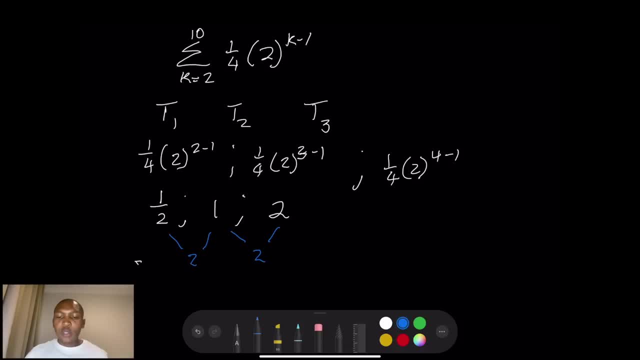 okay, so that simply means that if you take term three divided by term two, you get two, and you take term two divided by term one, that gives you two as well. all right, so first of all, uh, let's, uh just see there. so it means our a value. 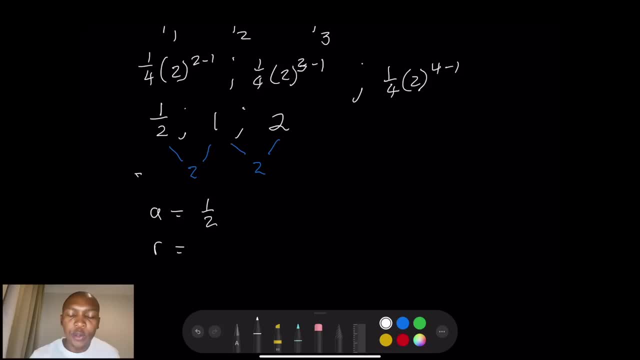 is one over two and it means our r value is um two. so in this particular case, because our r value is greater than one, you remember that. so for the geometric series, you've got a. you remember that. so for the geometric series, you've got a. you remember that. so for the geometric series, you've got a convergent and a divergent series. 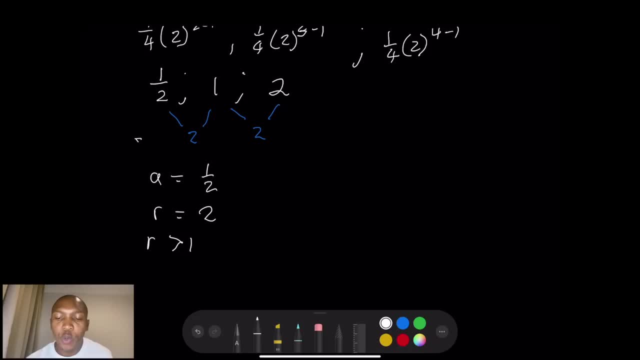 convergent and a divergent series, convergent and a divergent series, and of course it all depends on the value and of course it all depends on the value and of course it all depends on the value of r. so now we're looking for the sum. now 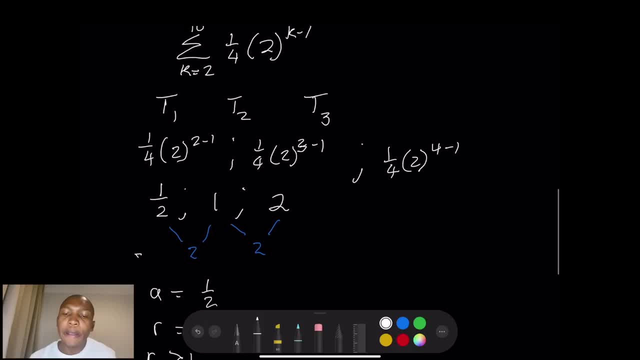 of r. so now we're looking for the sum now of r. so now we're looking for the sum. now, please note, we are taking from two till. please note we are taking from two till. please note, we are taking from two till ten. ten, okay, so how many terms is that? 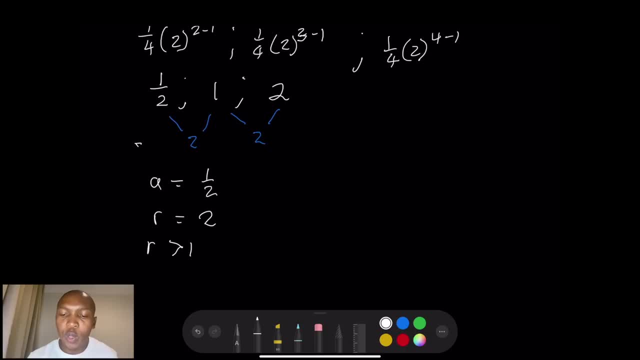 ten, ten, okay, so how many terms is that? ten, ten, okay, so how many terms is that? that will be nine terms. right so it? that will be nine terms. right so it. that will be nine terms. right, so it means that we're going to say s means that we're going to say s. 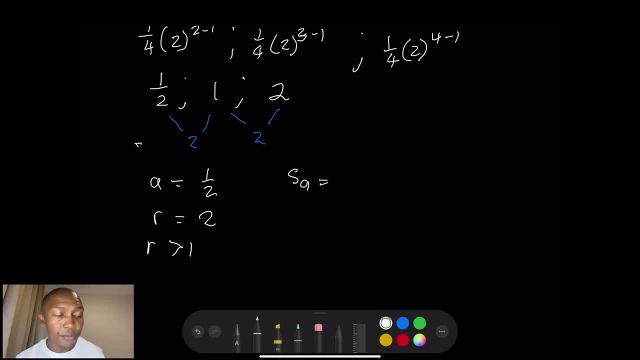 means that we're going to say s nine. okay, so you remember the formula nine. okay, so you remember the formula nine. okay, so you remember the formula: uh for the sum of your um. uh for the sum of your um. uh for the sum of your um. you know, if your um. 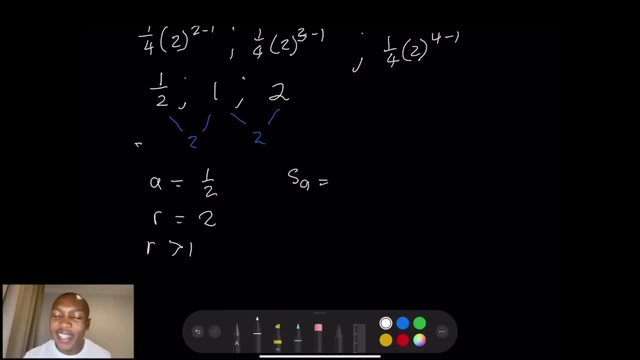 you know if your um. you know if your um. what do they call this? there's the name. what do they call this? there's the name. what do they call this? there's the name: geometric series. you know the name just: geometric series. you know the name just. 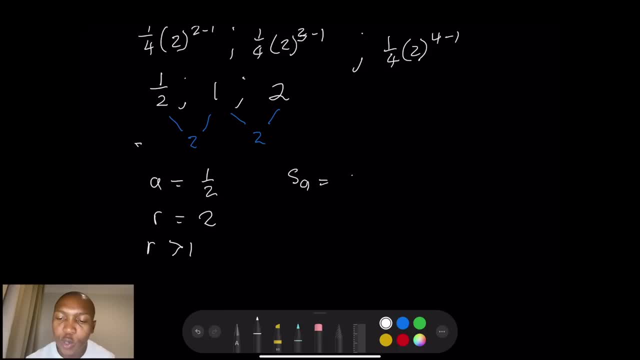 geometric series. you know the name just simply, simply, simply, slipped out of my mind. okay, so we're slipped out of my mind, okay, so we're slipped out of my mind, okay, so we're going to say this is a. going to say this is a. going to say this is a to the power, or rather a bracket, we've. 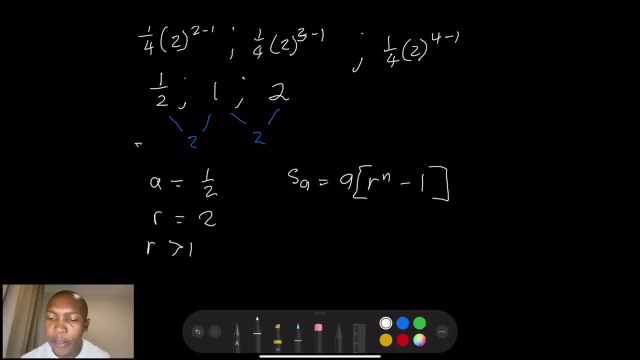 to the power, or rather a bracket. we've to the power, or rather a bracket. we've got r to the power n minus one. got r to the power n minus one. got r to the power n minus one. okay, divided by okay, divided by okay. divided by um r minus one. of course, this is for when. 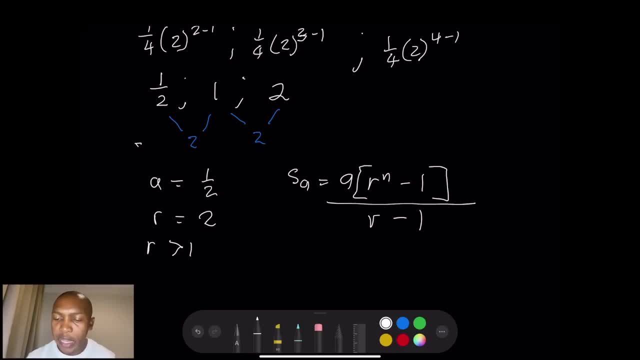 um r minus one. of course this is for when um r minus one. of course this is for when r is greater than one. it would be: r is greater than one. it would be r is greater than one. it would be expressed differently, expressed differently, expressed differently, and i'm not sure why. i wrote a there. 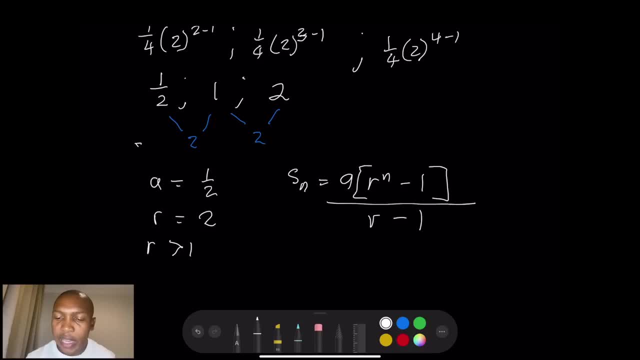 and i'm not sure why i wrote a there. and i'm not sure why i wrote a there instead of n, instead of n, instead of n. okay, so that's s? n. so we know we're okay. so that's s? n. so we know we're. 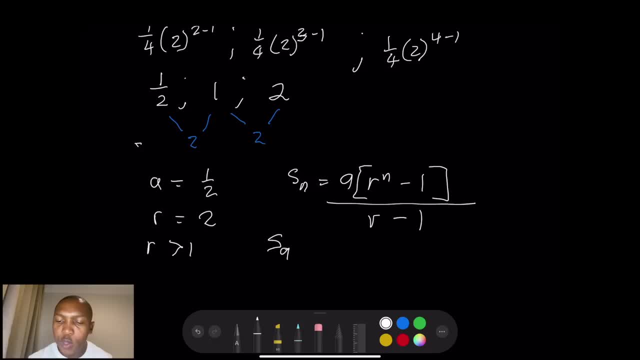 okay, so that's s n. so we know we're dealing with s. dealing with s. dealing with s nine, right, okay, so s nine. nine, right, okay, so s nine. nine, right, okay, so s nine. that is going to be a our a value is. that is going to be a our a value is. 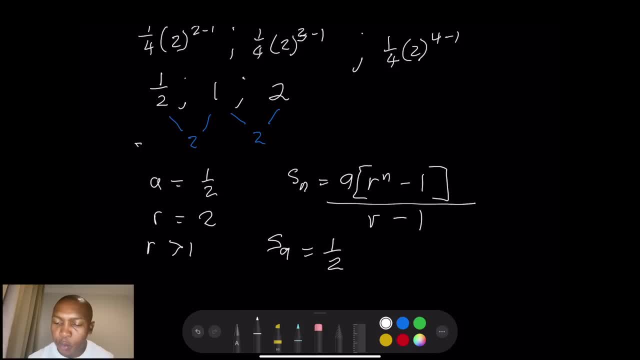 that is going to be a our a value is one over two, and i'm going to one over two and i'm going to one over two and i'm going to make those brackets uh to be different. make those brackets uh to be different. make those brackets uh to be different. okay. 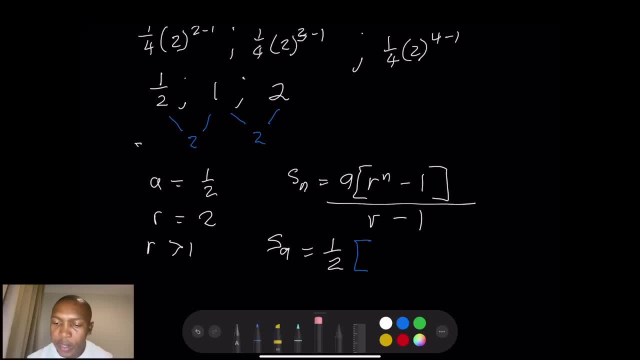 okay, okay, um, so that's r. um, so that's r. um, so that's r. so our r value is two. so our r value is two. so our r value is two. uh, our value is two. okay, let me just use. uh, our value is two. okay, let me just use. 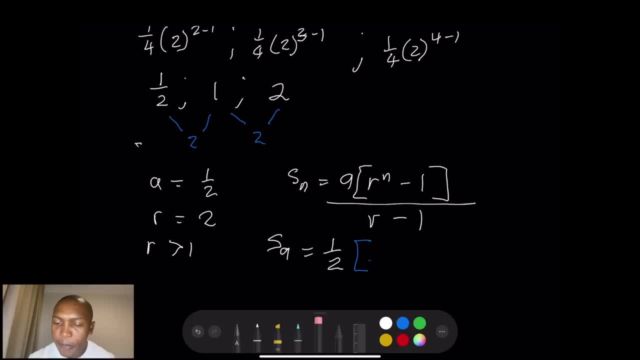 uh, our value is two. okay, let me just use a, a, a. let me stick to white again. let me stick to white again. let me stick to white again. all right, yeah, having to toggle with. all right, yeah, having to toggle with. all right. yeah, having to toggle with these colors. 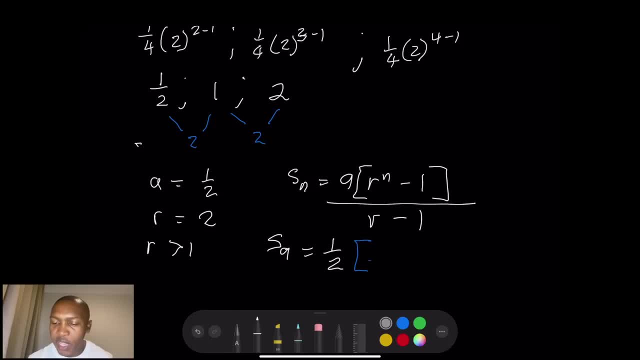 these colors, these colors. uh is a bit daunting, but we'll get there. uh is a bit daunting, but we'll get there. uh is a bit daunting, but we'll get there. okay, so this is going to be two. okay, so this is going to be two. okay, so this is going to be two. uh, to the power now. please remember in. 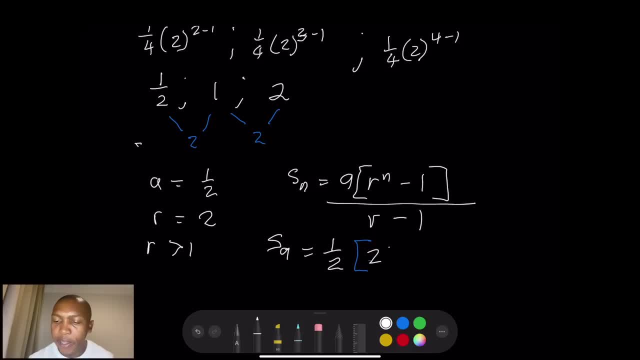 uh to the power now, please remember. in uh to the power now. please remember in this case. we said this case. we said this case. we said n? n is nine okay, so nine. n? n is nine okay, so nine. n n is nine okay, so nine minus one okay, and i'm going to close. 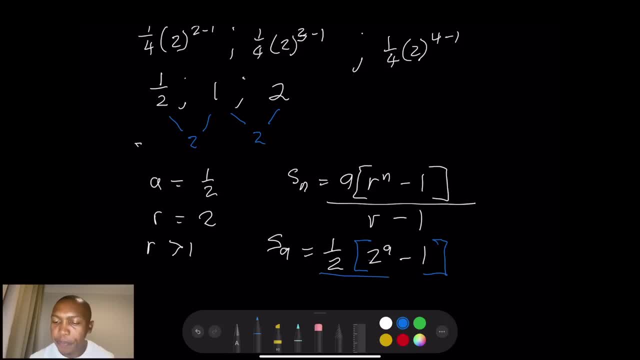 minus one, okay, and i'm going to close minus one, okay, and i'm going to close that bracket, that bracket, that bracket, divided by, divided by, divided by, in this particular case, in this particular case, in this particular case, divided by. again, this is going to be r. 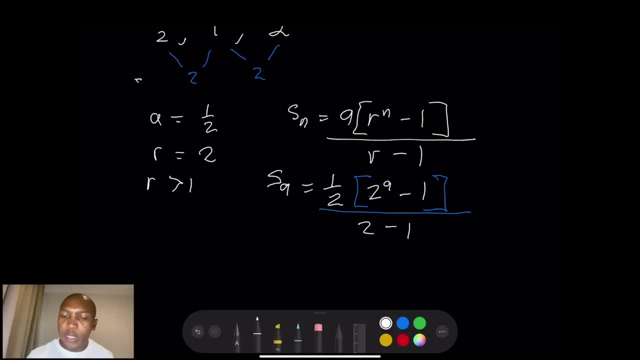 divided by again, this is going to be r. divided by again, this is going to be r, which is our two, which is our two, which is our two, minus one: all right quickly, uh. if we work minus one, all right quickly, uh, if we work minus one, all right quickly, uh, if we work that out. let's find out what that is. 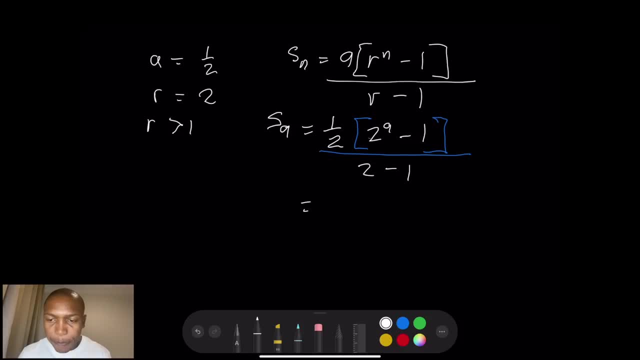 that out, let's find out what that is. that out, let's find out what that is. so this is going to be one over two. so this is going to be one over two. so this is going to be one over two. okay, multiplied by two to the power nine. 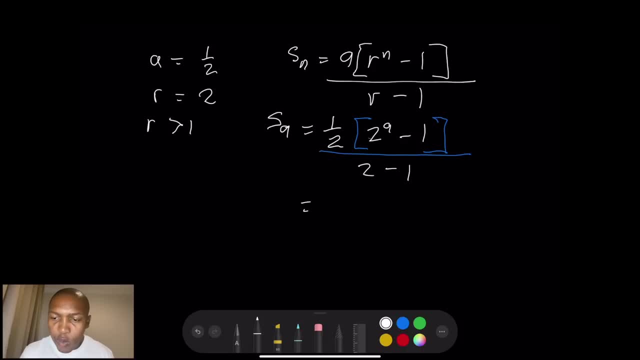 okay, multiplied by two to the power nine: okay, multiplied by two to the power nine, minus minus minus one. okay, all right. two minus one, one, okay, all right. two minus one. one. okay, all right. two minus one is one. so, um, that gives me, is one. so, um, that gives me. 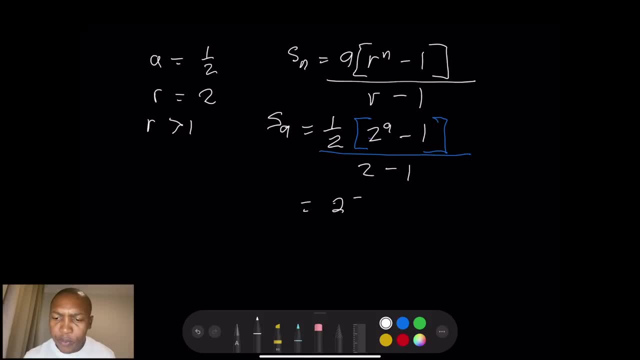 is one. so, um, that gives me a value of two hundred and a value of two hundred and a value of two hundred and fifty five, fifty five, fifty five, point five, so point five, so point five. so some, some, some. the first nine terms is going to be 255.5. 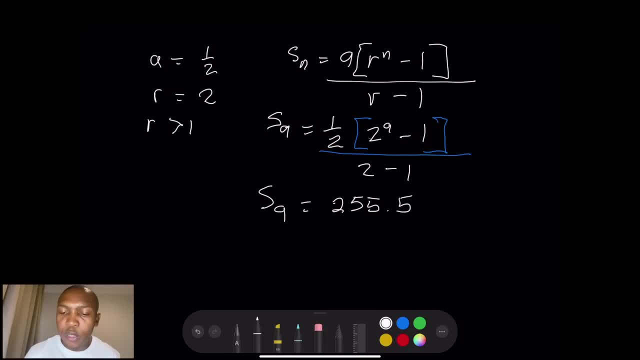 the first nine terms is going to be 255.5. the first nine terms is going to be 255.5. all right, you can please verify that, for all right. you can please verify that, for all right. you can please verify that for me and just make sure that we are all on. 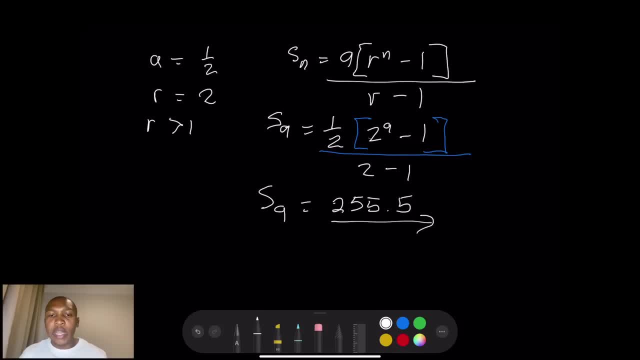 me and just make sure that we are all on me and just make sure that we are all on the same page. the same page, the same page, and essentially that is how we would get and essentially that is how we would get and essentially that is how we would get our answer. all right, i hope that's been. 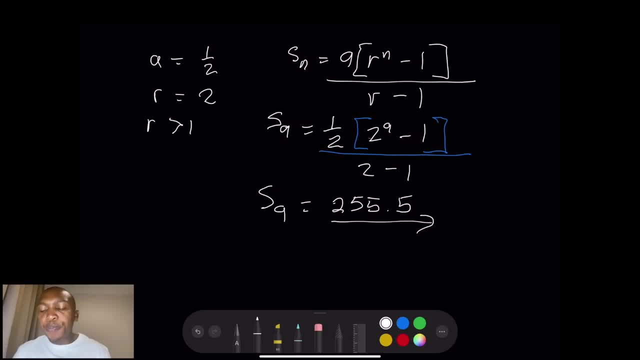 our answer all right. i hope that's been our answer all right. i hope that's been understandable, understandable, understandable. so just the last thing that i want us to, so, just the last thing that i want us to, so, just the last thing that i want us to do, i want us to take a series. 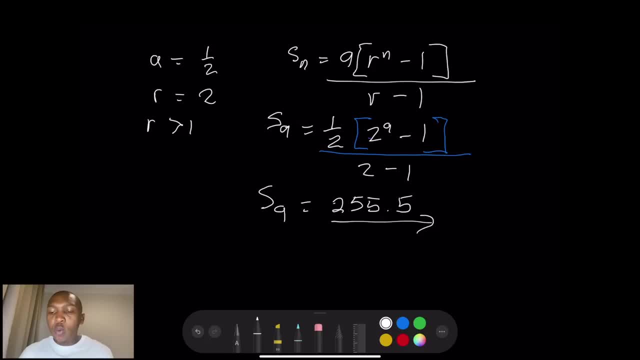 do i want us to take a series? do i want us to take a series, um, um. what happens in a series, um, um. what happens in a series, um, um. what happens in a series when we are given um, you know the. when we are given um, you know the. 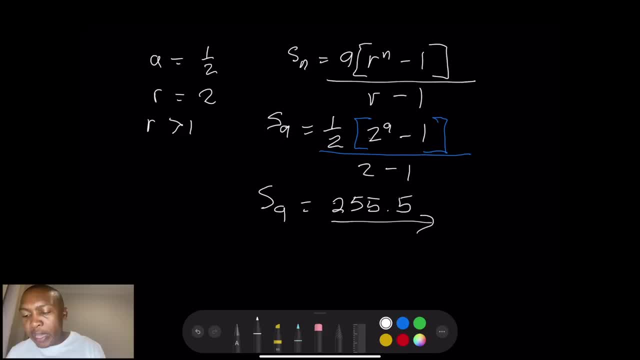 when we are given, um, you know the series and we want to express it series, and we want to express it series and we want to express it as a sigma in sigma notation. okay, let's, as a sigma in sigma notation. okay, let's, Let's look at that quickly. All right, So quickly, let's look at this. 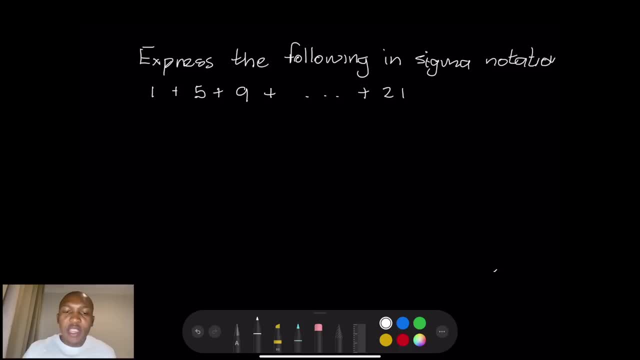 They say: express the following in sigma notation: OK, my board got cut there, So that's 1 plus 5 plus 9 up until 21.. All right, So the first thing that we're going to do is let's find out first. you know what type of a sequence is it? 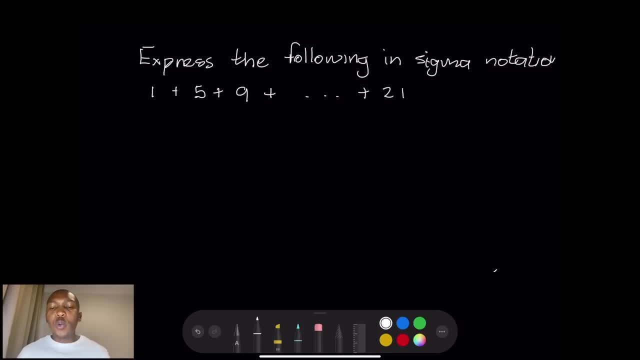 OK, Or rather a series. it is OK, Yeah, So in this particular case, if I look at that, the first term, So that's going to be T1.. That's T2.. That's T3. And we don't know what T that is, but we'll get to that. 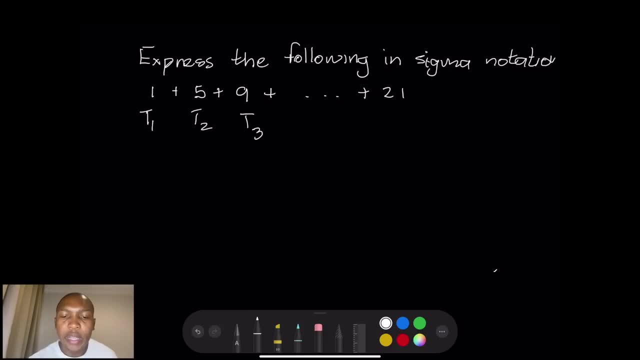 So if I look at T2 minus T1,, that's 5 minus 4 minus 1, which is equals to 4.. So, and that tells me that the difference between the first and the second term is 4.. But if I look at term 3 minus term 2, again, that's 9 minus 5, which also gives me 4.. 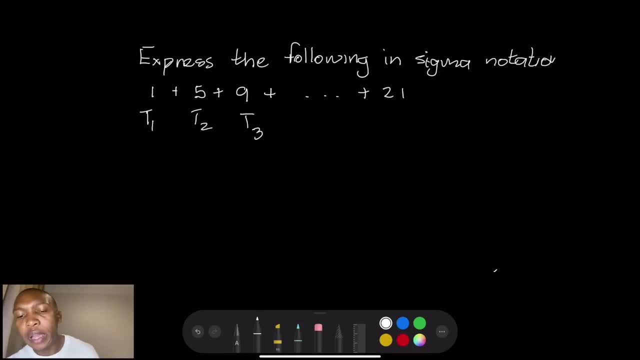 So that's kind of tells me that this is a an arithmetic sequence. OK, so now we're going to look for the sigma notation of it, But first of all it means that our A value is 1 and our D is 4.. 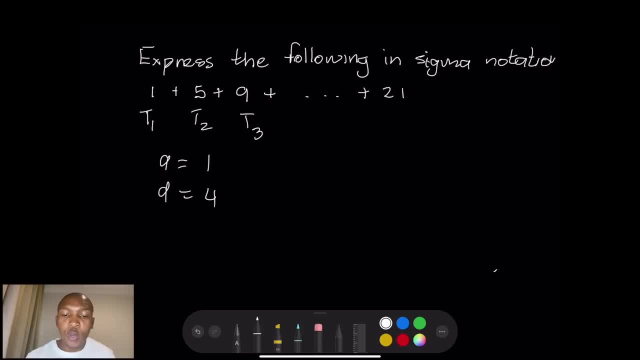 OK, so let's find the general expression. So that's where we, That's what we'd always do. So find the general expression. So the general expression is T. N is equal to Now, please remember, for the arithmetic sequence, that's A plus N minus 1 times D. 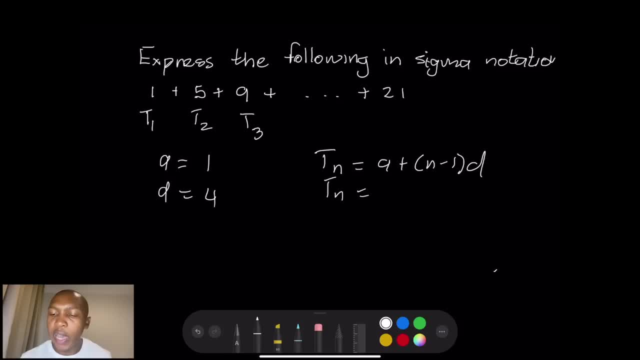 OK, so let's substitute for everything that we know. So T N is A, which is 1 plus, in this case N minus 1.. N minus 1 multiplied by. So we're going to substitute that in there, All right, and please remember, we're going to substitute into both of those. 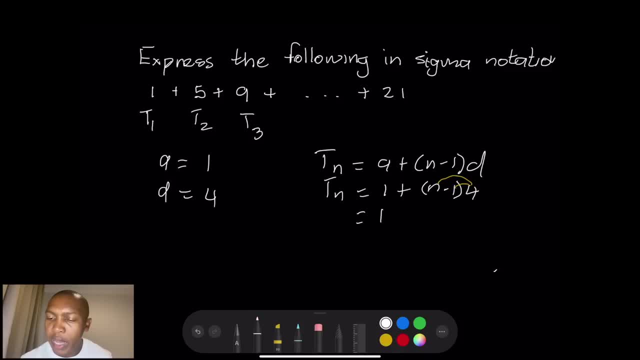 So now that becomes 4 times N, That becomes 4 N minus 4 times 1.. And remember it's positive times, a negative, That's going to be minus 4.. So our general expression: There is going to simply be 4 N minus 3.. 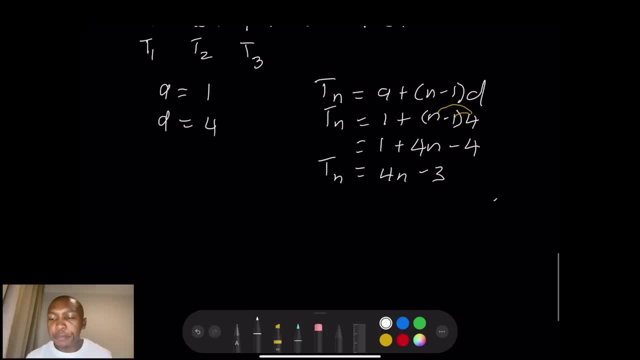 So that is our general expression. right For the sequence. Now, in this particular case, we know we're going to start at term 1.. If you take that expression, you know, let's see if I substitute 1.. OK, in there that's 4 times 1 minus 3.. 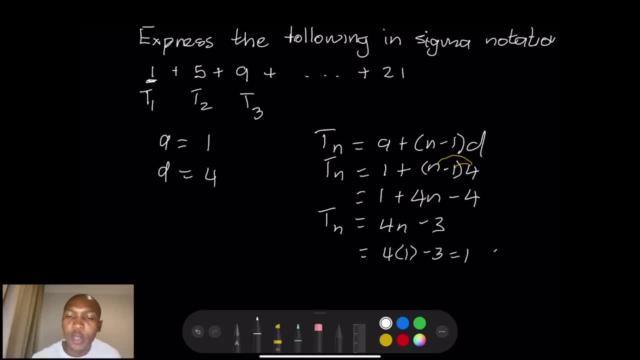 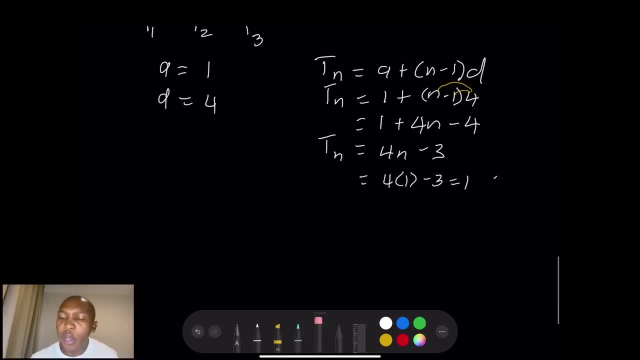 That definitely gives me 1, which is the first. OK, but now I want to know which term is 21.. So let's find that out quickly. So which term actually gives us 21?? So T, N, which is 4 N minus 3, is equal to 21.. 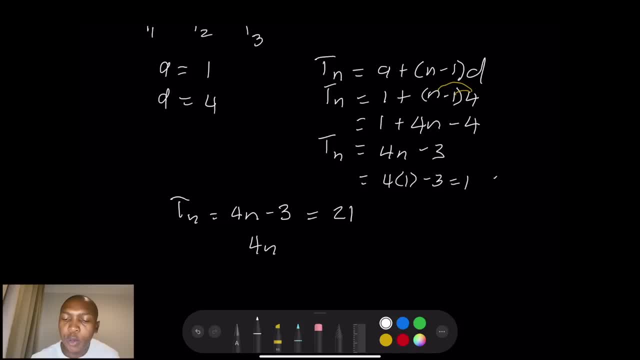 So we're going to say this is 4 N. I'm going to just take 3 to the other side, In this case 21.. Minus, OK. in this case it would be plus 3. So that would give us 24.. 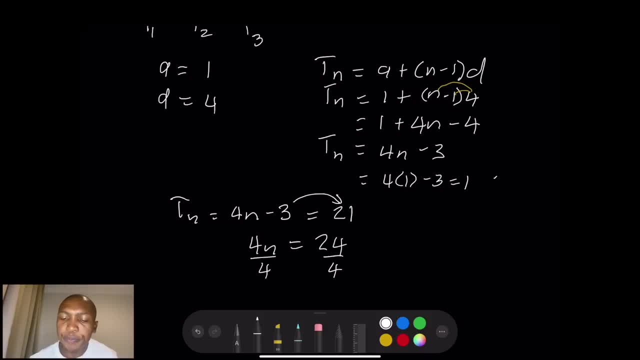 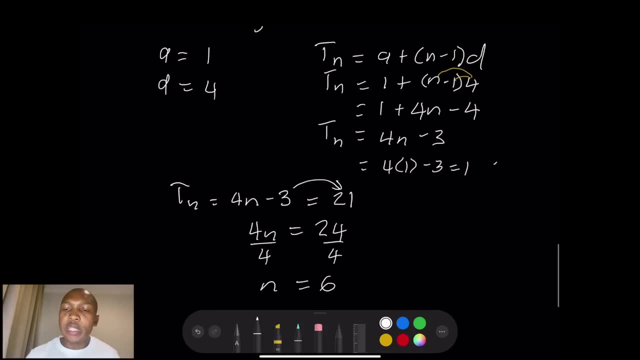 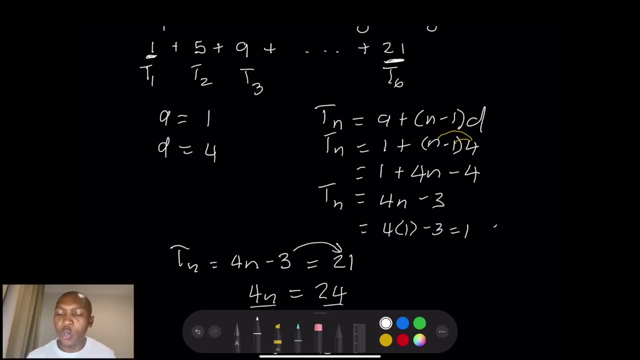 And if I divide both sides by 4.. OK, so N would be equal to 6.. OK, so, which means that you know the sixth term here, the sixth term is actually equal to 21.. Yeah, So how do I write this as a sigma? 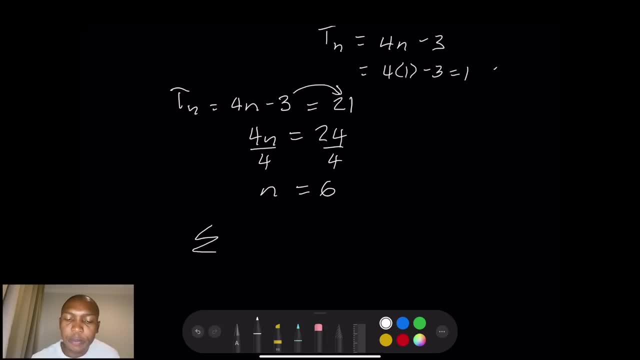 Sima notation. all I'm simply going to say is: OK, please forgive me. You know I keep trying to write with different colors because I wanted to kind of be visually appealing so that it just doesn't become bland and monotone. 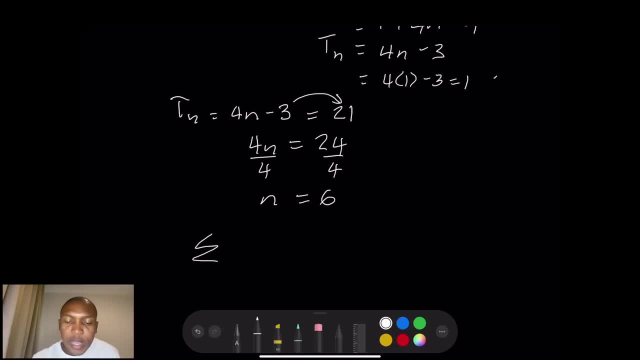 But of course, as I said, we'll get there All right. So in this case it's going to be N equals 1 up until 6.. And our general expression, we said that's going to be 4N minus 3.. 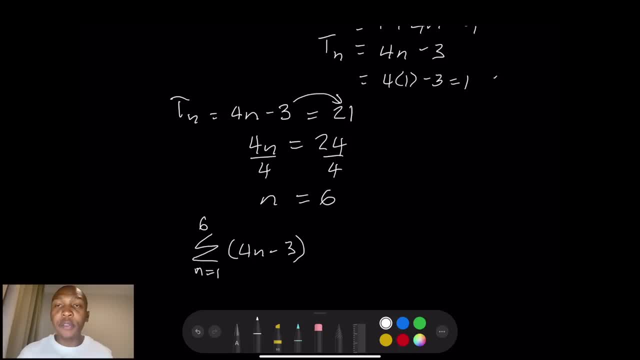 Nothing wrong if you wanted to express it as K or whatever the other you have in this case. Remember, when you change it there, you also have to change it there. All right, And that is how you write that series in sigma notation.